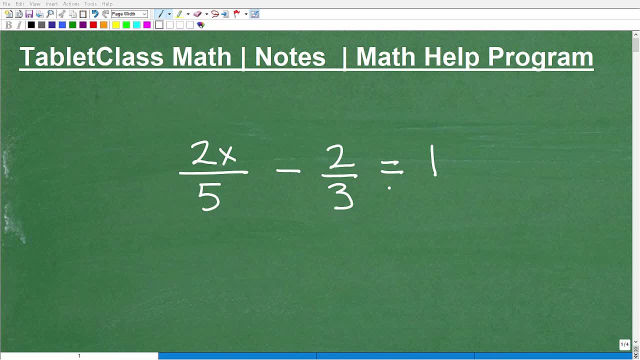 And so what? you know what's kind of the best path to handle an equation that involves fractions- Basic algebra equation. There's a couple different things here that we can do to help us out, But I'm going to teach you here is probably the most well, in my opinion, probably the easiest- approach to doing a problem like this. 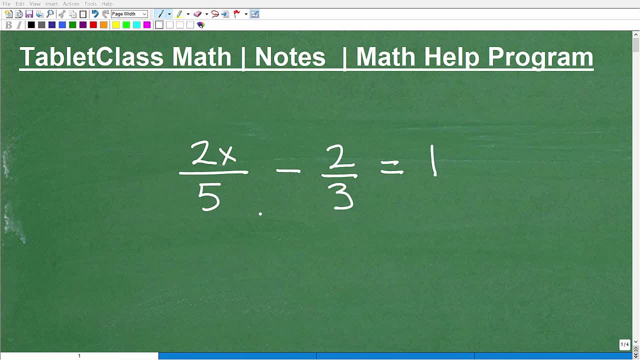 So you definitely want to stick around, because solving equations with fractions in algebra comes up quite frequently. Okay, unfortunately, you know, all your equations aren't going to be like you know: 3y equals 9.. Okay, you start off learning. 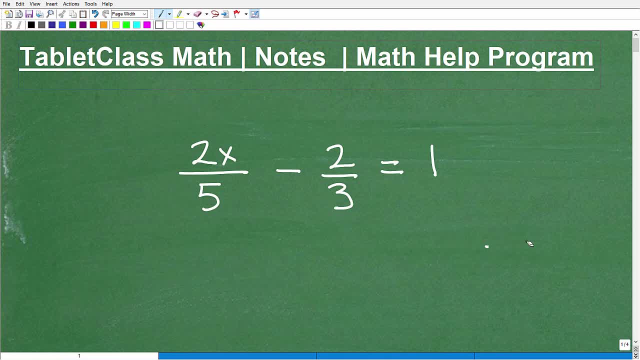 You start off learning equations with things like this, But then, of course, they get much more complex. All right, so, with that being said, I'm going to go ahead and get into this and teach you everything you need to know about dealing with these fraction equations. 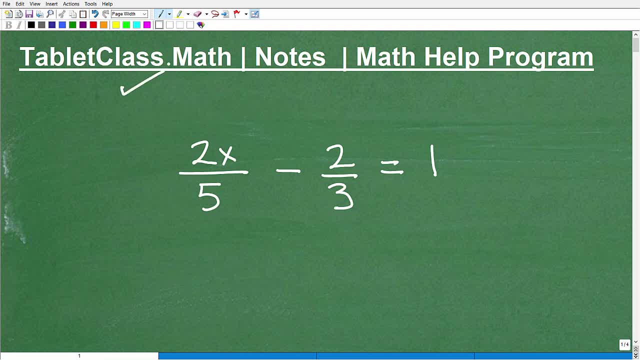 But first let me go ahead and introduce myself. My name is John. I'm the founder of Tablet Class Math. I'm also a middle and high school math teacher And over many years I've constructed what I like to believe is one of the most robust, comprehensive online video-based math help programs there is. 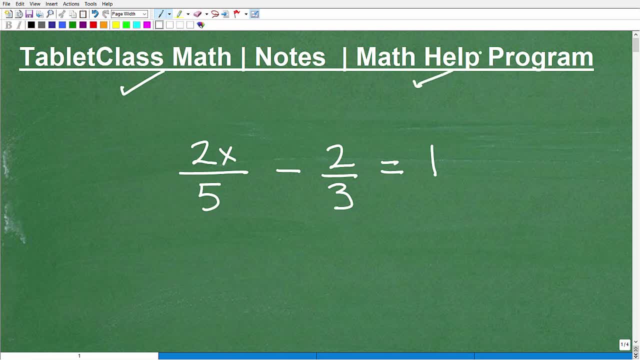 It's taken me literally years and years, and years. So if you need to take a full math course or you're in a math course and need super comprehensive video-based lessons, or if you want to see thousands of problems solved via video-based explanation, step-by-step- 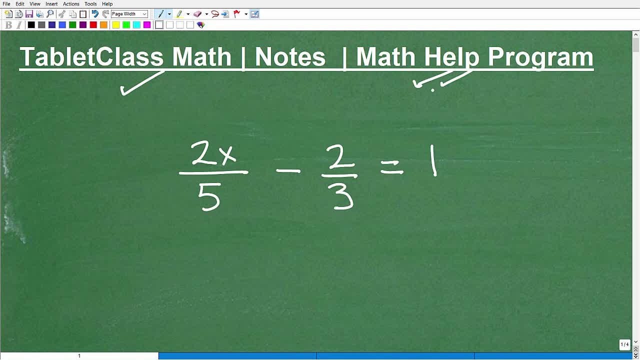 then you definitely want to check out my math help program. I'm going to leave a link to that in the description of this video. Also, if you've been following me on YouTube, you should know that I strongly emphasize note-taking. Okay. 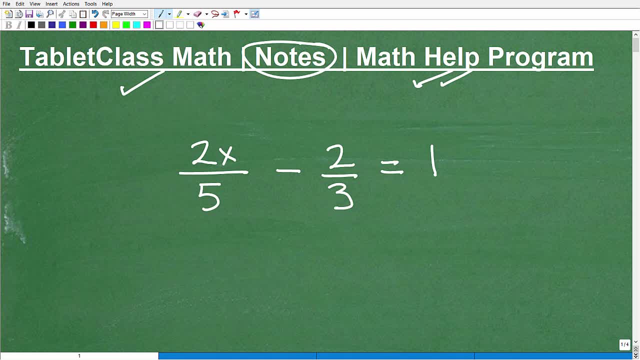 Okay, The quality of your notes Okay, And this comes from decades of teaching mathematics- Your notes is one of the best indicators I know of from my personal experience for students. Basically, here's what I'm trying to say: Those students who do great in math have great notes. 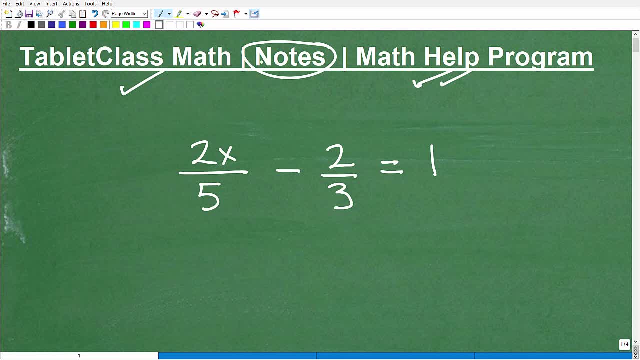 Okay And it kind of reverses: true, You take great notes, you're going to do very well in math. So if you want to kind of get a sense of like, hey, how well you're doing in math, if you're doing the right things, look at your notes. 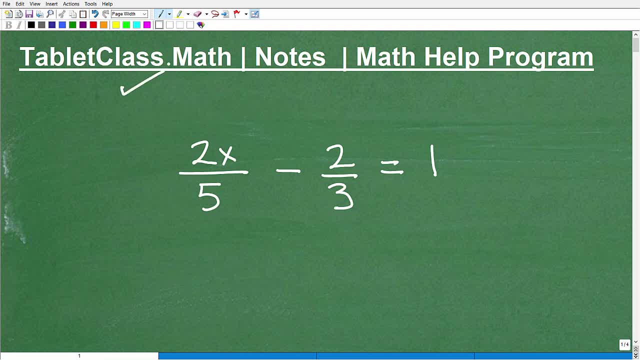 But first let me go ahead and introduce myself. My name is John. I'm the founder of Tablet Class Math. I'm also a middle and high school math teacher And over many years I've constructed what I like to believe is one of the most robust, comprehensive online video-based math help programs there is. 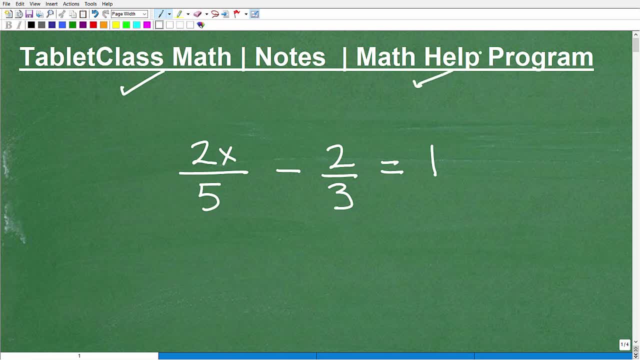 It's taken me literally years and years, and years. So if you need to take a full math course or you're in a math course and need super comprehensive video-based lessons, or if you want to see thousands of problems solved via video-based explanation, step-by-step- 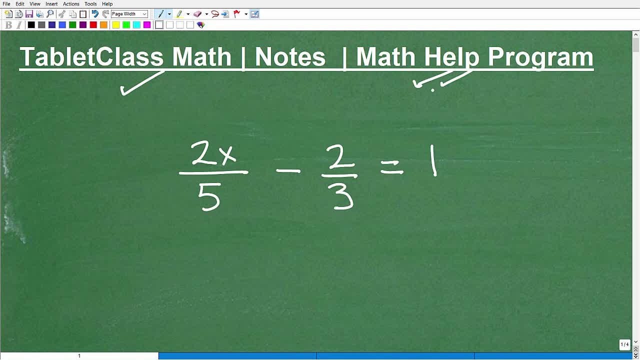 then you definitely want to check out my math help program. I'm going to leave a link to that in the description of this video. Also, if you've been following me on YouTube, you should know that I strongly emphasize note-taking. Okay. 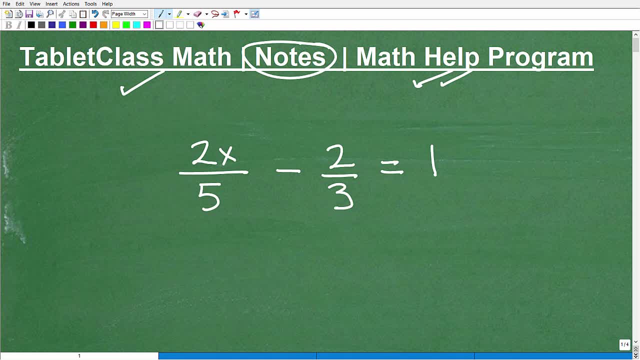 Okay, The quality of your notes Okay, And this comes from decades of teaching mathematics- Your notes is one of the best indicators I know of from my personal experience for students. Basically, here's what I'm trying to say: Those students who do great in math have great notes. 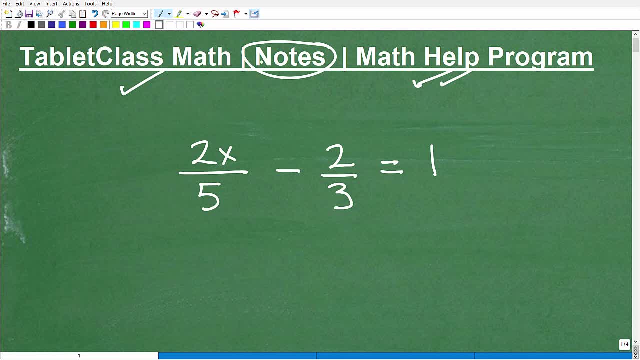 Okay And it kind of reverses: true, You take great notes, you're going to do very well in math. So if you want to kind of get a sense of like, hey, how well you're doing in math, if you're doing the right things, look at your notes. 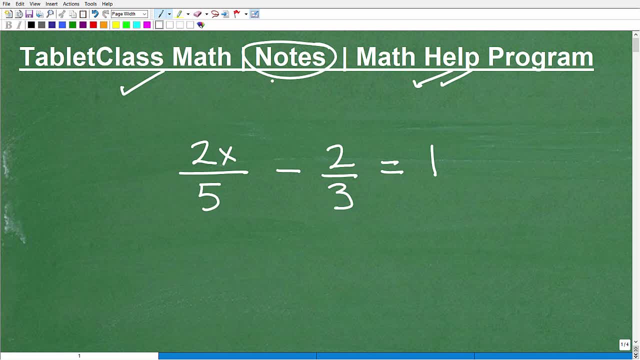 Okay, Could you give your notes to somebody else And could that person learn math from your notes? Your notes should be of that quality, Okay. So if they're not, it's certainly understandable, because a lot of students, you know, don't work hard enough on their notes. 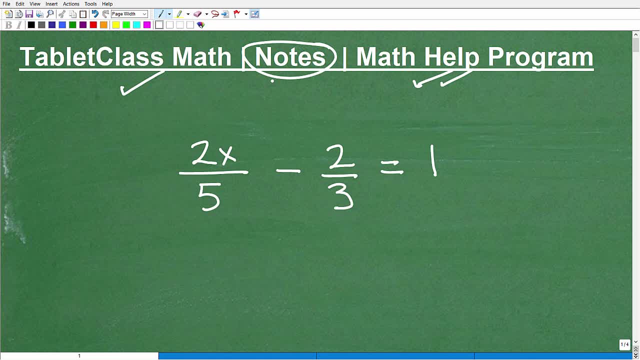 It is a skill. Okay, So I got some other videos on note-taking. All right, Importance of note-taking, But I like to emphasize this in all the videos I do Now. with that being said, you definitely need something to study from still. 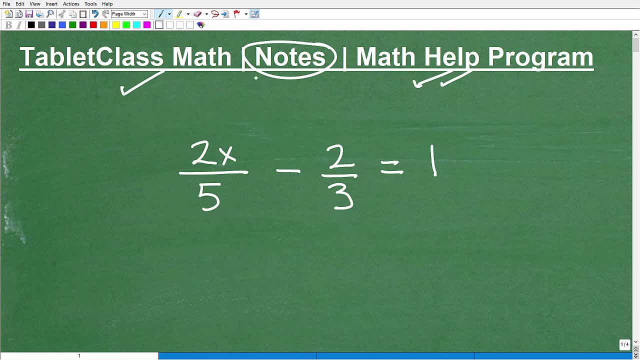 So I offer notes. I'm going to leave a link to my notes in the description of this video. Those would include pre-algebra. algebra one, geometry. algebra two, trigonometry. So if you need notes- which you do need notes, if your notes aren't up to speed, you can check out my notes there. 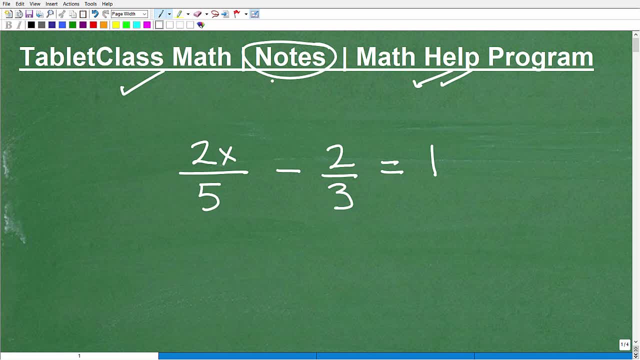 Okay, Could you give your notes to somebody else And could that person learn math from your notes? Your notes should be of that quality, Okay. So if they're not, it's certainly understandable, because a lot of students, you know, don't work hard enough on their notes. 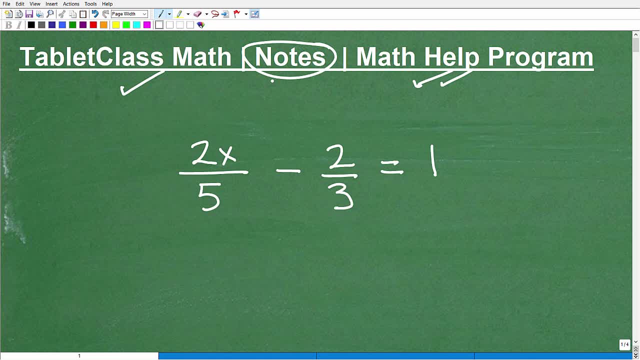 It is a skill. Okay, So I got some other videos on note-taking. All right, Importance of note-taking, But I like to emphasize this in all the videos I do Now. with that being said, you definitely need something to study from still. 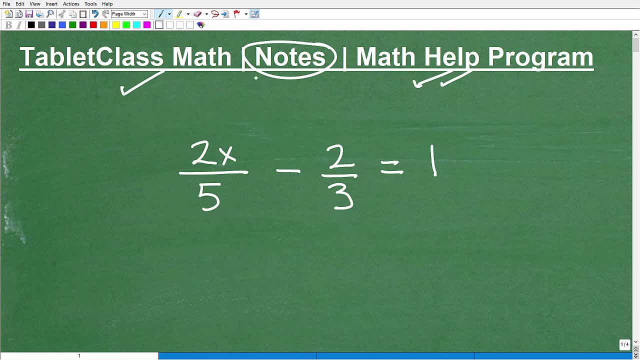 So I offer notes. I'm going to leave a link to my notes in the description of this video. Those would include pre-algebra. algebra one, geometry. algebra two, trigonometry. So if you need notes- which you do need notes, if your notes aren't up to speed, you can check out my notes there. 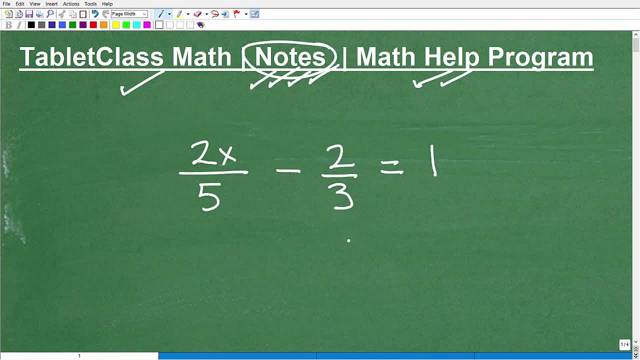 All right, So let's get into this problem. Now, of course, you know we're dealing with a basic equation, a basic algebra equation, And let's just Think about this just in more simpler terms. So let's get rid of some fractions and let's just think what if I just had the equation two? 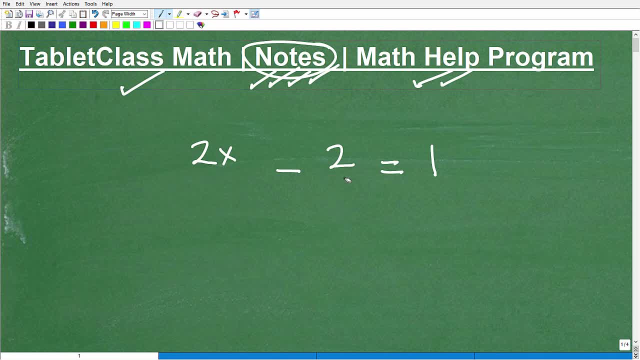 Well, let's just erase this, Right. Let's just erase this like so: Okay, Just get rid of the fractions Now to be able to handle a fraction equation. my question to you is: could you handle this basic equation right here? 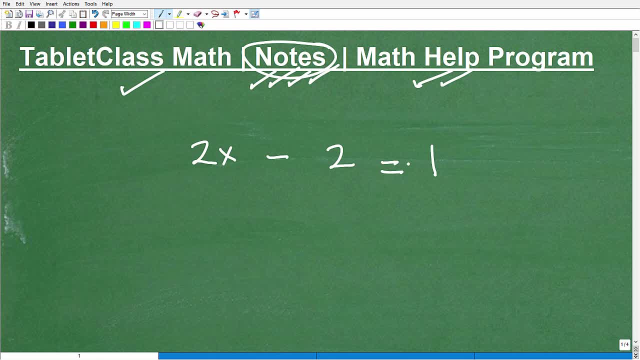 Okay, This is what we would call a two-step equation in algebra. So before you can handle equations with fractions, you got to be able to handle the basic stuff Right. So let's go ahead and just review how to handle something like this. 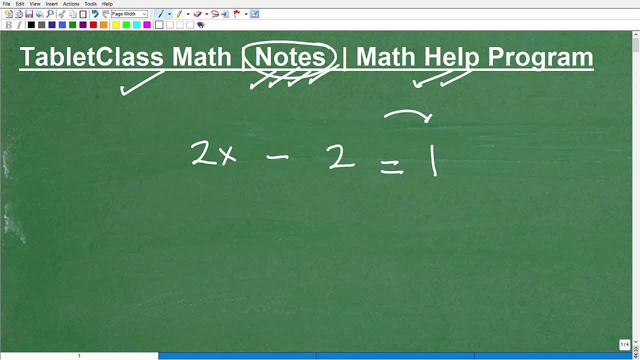 First thing you want to do is to move all your numbers to this side of the equation and have all your variables on this side of the equation. So the way I'm going to do that is I'm going to add two to both sides of the equation, like so. 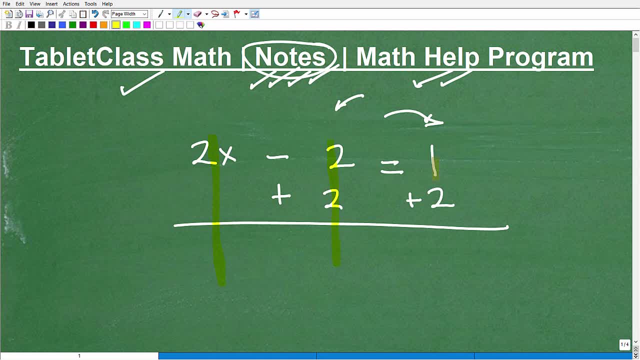 Okay, And then you want to kind of conceptually add down like so: All right, Now this is. there's other formats to solve equations. One I'm showing you here is definitely by far the most common And it's the best way to kind of structure your work. 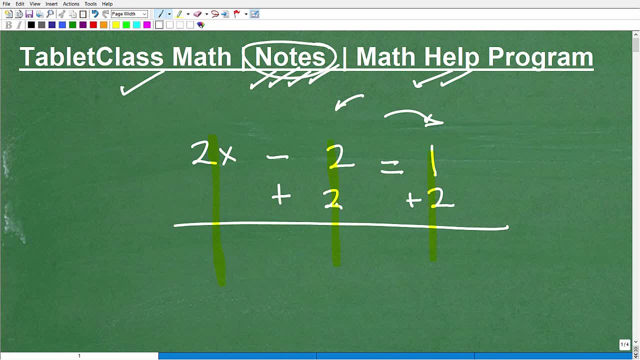 So when I add down 2x plus, nothing is 2x Negative. 2 plus 2 is 0. So I'm left with 2x over here, And then 1 plus 2 is 3.. And now that's my first step. 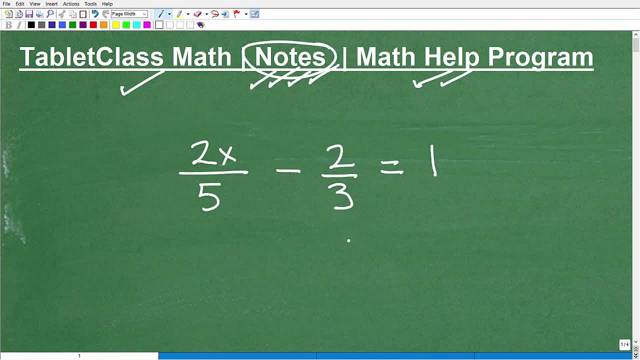 All right, So let's get into this problem. Now, of course, you know we're dealing with a basic equation, a basic algebra equation, And let's just Think about this just in more simpler terms. So let's get rid of some fractions and let's just think what if I just had the equation two? 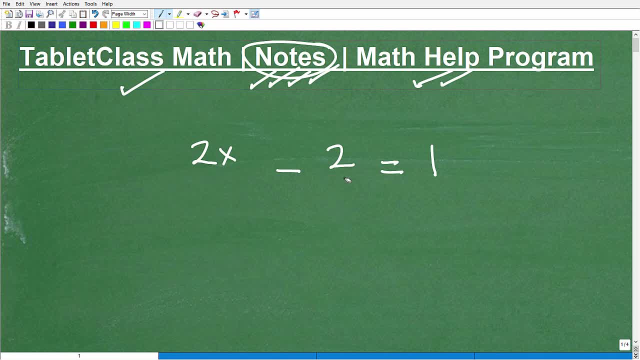 Well, let's just erase this, Right. Let's just erase this like so: Okay, Just get rid of the fractions Now to be able to handle a fraction equation. my question to you is: could you handle this basic equation right here? 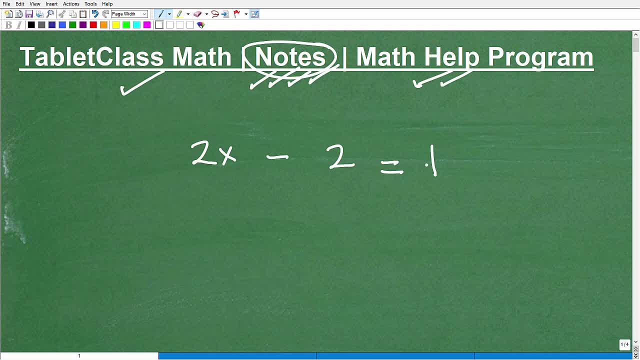 Okay, This is what we would call a two-step equation in algebra. So before you can handle equations with fractions, you got to be able to handle the basic stuff Right. So let's go ahead and just review how to handle something like this. 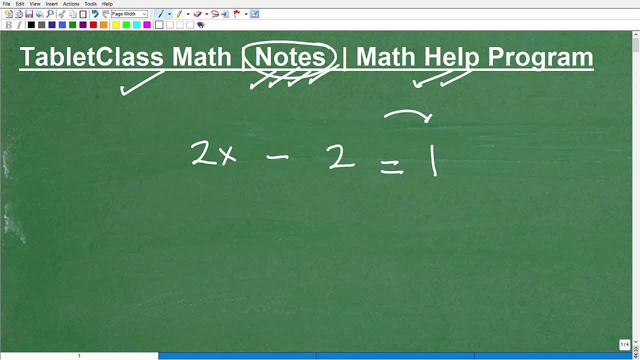 First thing you want to do is to move all your numbers to this side of the equation and have all your variables on this side of the equation. So the way I'm going to do that is I'm going to add two to both sides of the equation, like so. 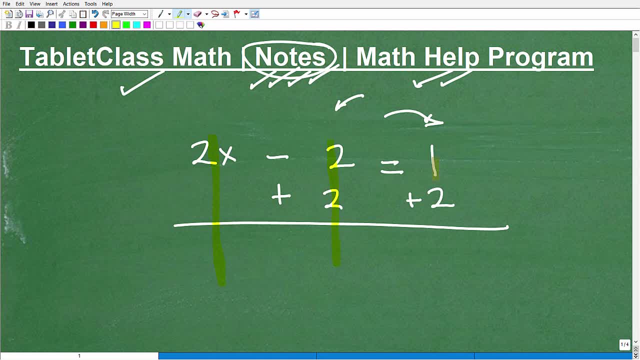 Okay, And then you want to kind of conceptually add down like so: All right, Now this is. there's other formats to solve equations. One I'm showing you here is definitely by far the most common And it's the best way to kind of structure your work. 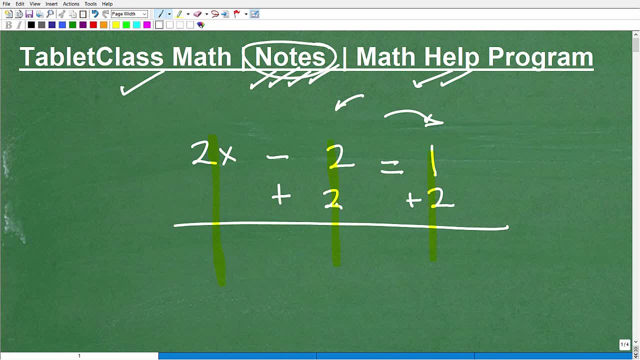 So when I add down 2x plus, nothing is 2x Negative. 2 plus 2 is 0. So I'm left with 2x over here, And then 1 plus 2 is 3.. And now that's my first step. 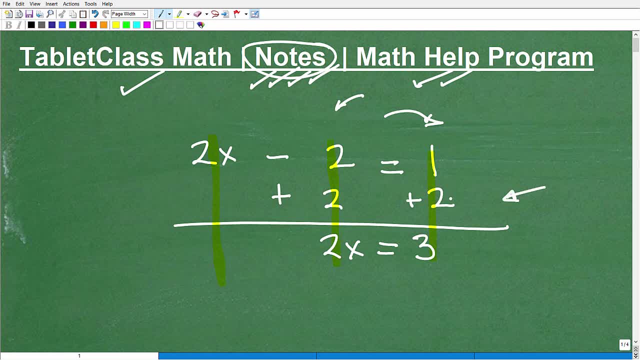 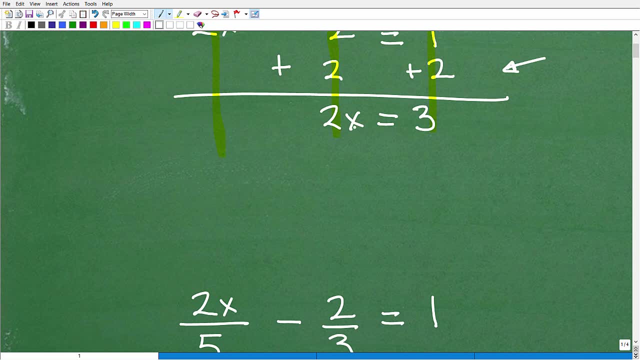 Okay, So that's. my first step was to get all my numbers on the right-hand side and have all my variables here on the left-hand side. Okay, So now? what do I do here? Of course I have the problem down this fraction problem. 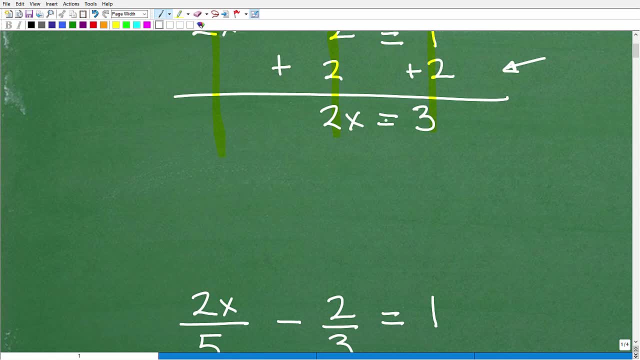 We're going to do here in a second. Don't worry about that. Let's go ahead and finish up with this guy. So 2x equals 3.. What do I do to solve for x? Well, you got it. I got to divide both sides of the equation by 2.. 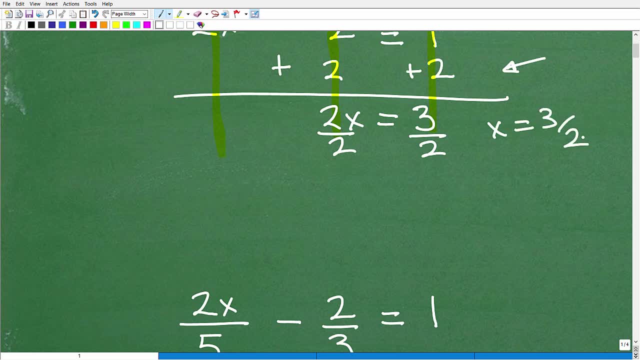 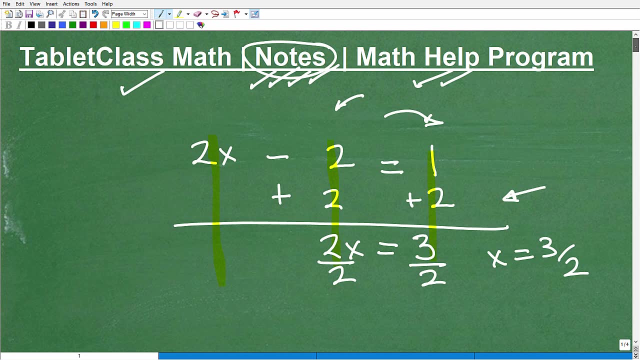 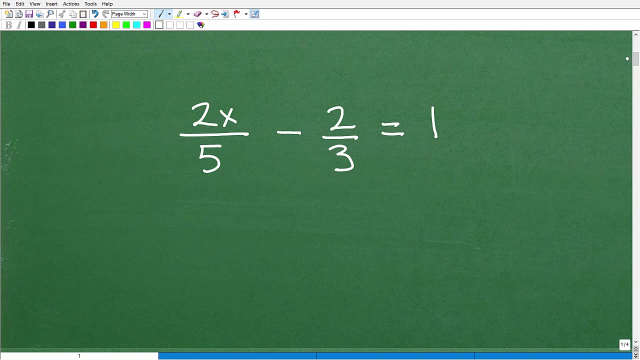 So x is equal to 3 halves. Okay, So if you're comfortable with- you know- that level of difficulty and basic algebra problems, then we can talk about something more interesting like this. All right, So a couple of different things you can do here. 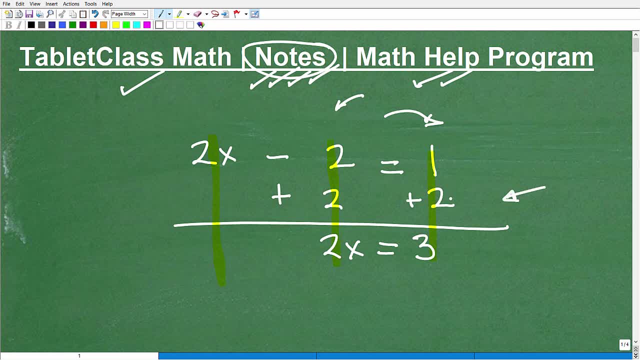 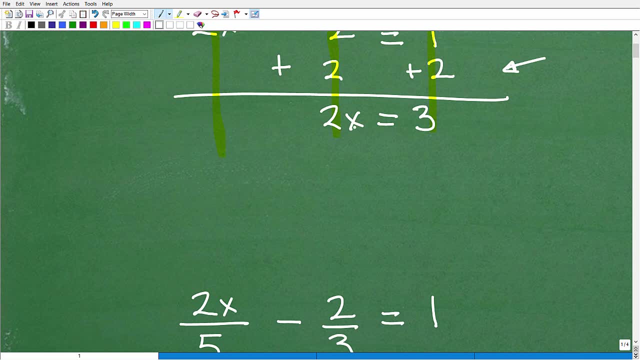 Okay, So that's. my first step was to get all my numbers on the right-hand side and have all my variables here on the left-hand side. Okay, So now? what do I do here? Of course I have the problem down this fraction problem. 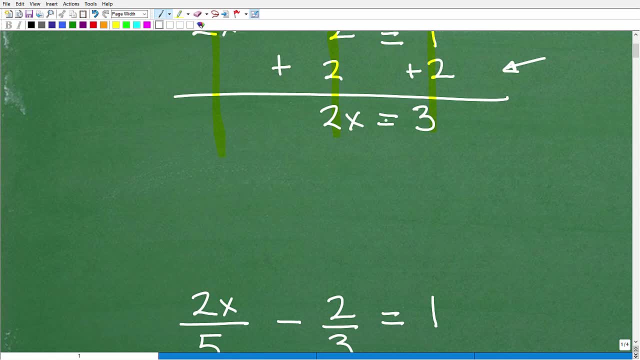 We're going to do here in a second. Don't worry about that. Let's go ahead and finish up with this guy. So 2x equals 3.. What do I do to solve for x? Well, you got it. I got to divide both sides of the equation by 2.. 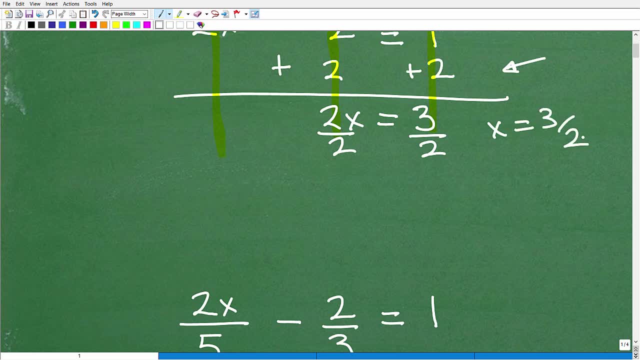 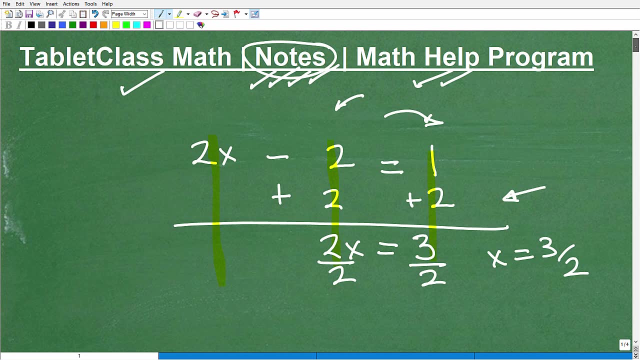 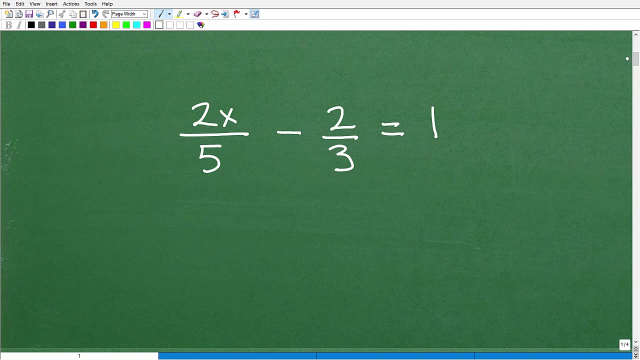 So x is equal to 3 halves. Okay, So if you're comfortable with- you know- that level of difficulty and basic algebra problems, then we can talk about something more interesting like this. All right, So a couple of different things you can do here. 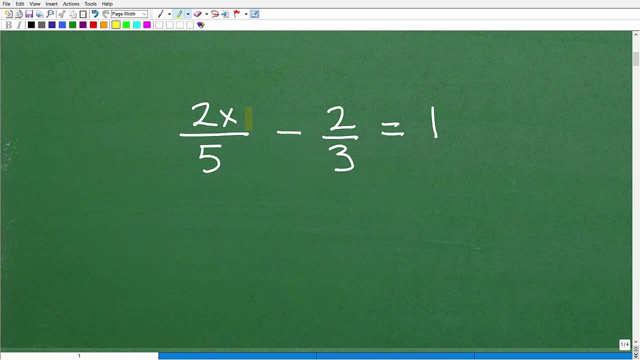 All right, Let's just look at kind of analyze what's going on. So I have my variable over here. Okay, So this is 2x over 5.. So 2x over 5. You can think of this as the term 2 fifths times x their equivalent. 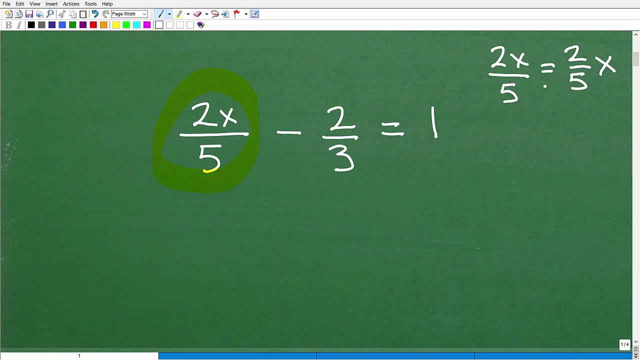 Okay, So these two are the same thing. Okay, So, if that helps you, you could be like: okay, I could. you know, that's 2 fifths times x minus something. So I have a number. It's in fraction form, but I have to move this over here like that. 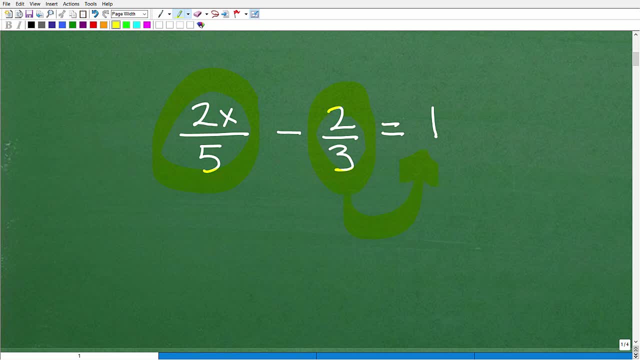 Right. So I'd have to add 2 thirds to both sides, And then I kind of follow the same steps as we did before. Now you could do that Right. There's nothing that says that you can't, So you can go like this: 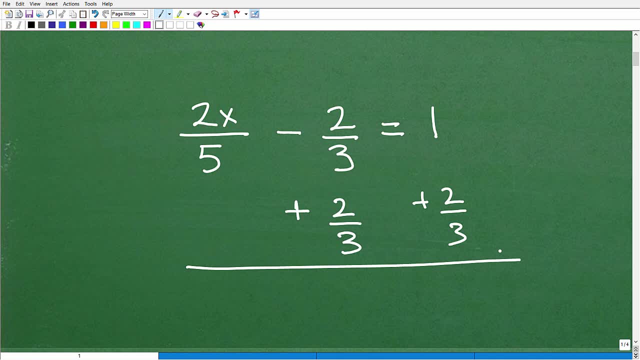 All right, And we can do all the number crunching and 1 plus 2 thirds, So then we'd end up with 2 fifths x over here And then we have 1 plus 2 thirds is 1 and 2 thirds. 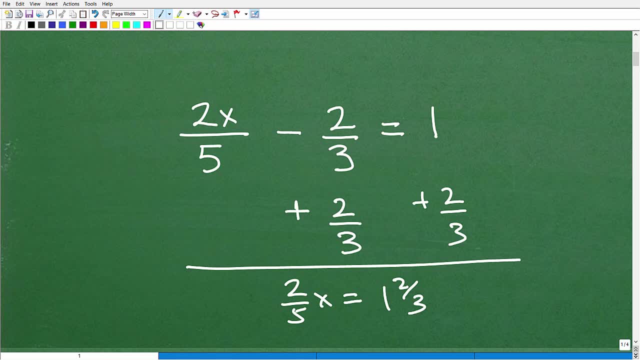 And we can kind of go from that route And then we can kind of solve. You need to know how to do the problem in that manner as well, But what I'm going to show you here is just a way that we can just kind of more cleanly, more efficiently do this problem. 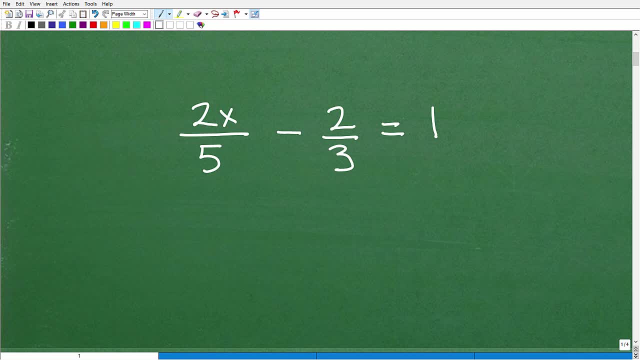 Okay, This is the way I'm going to teach my students, after I taught them more the long way. Okay, All right. So first of all, I'm like you. I don't want to be dealing with Fractions, Okay. 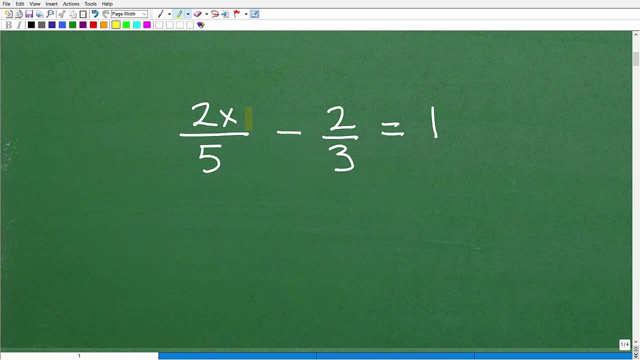 All right, Let's just look at kind of analyze what's going on. So I have my variable over here. Okay, So this is 2x over 5.. So 2x over 5. You can think of this as the term 2 fifths times x their equivalent. 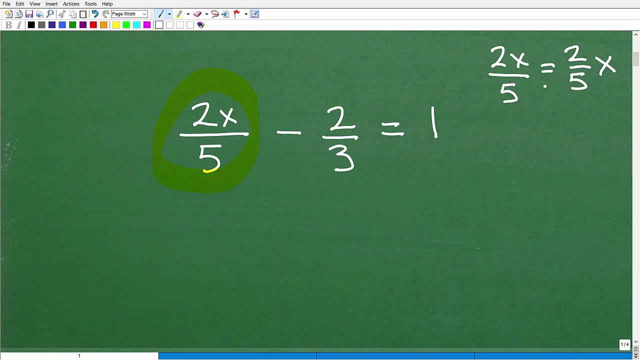 Okay, So these two are the same thing. Okay, So, if that helps you, you could be like: okay, I could. you know, that's 2 fifths times x minus something. So I have a number. It's in fraction form, but I have to move this over here like that. 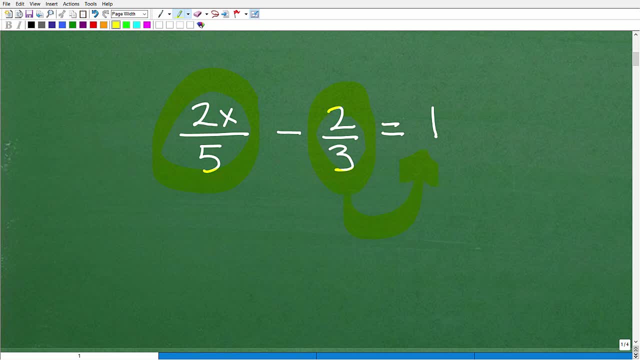 Right. So I'd have to add 2 thirds to both sides, And then I kind of follow the same steps as we did before. Now you could do that Right. There's nothing that says that you can't, So you can go like this: 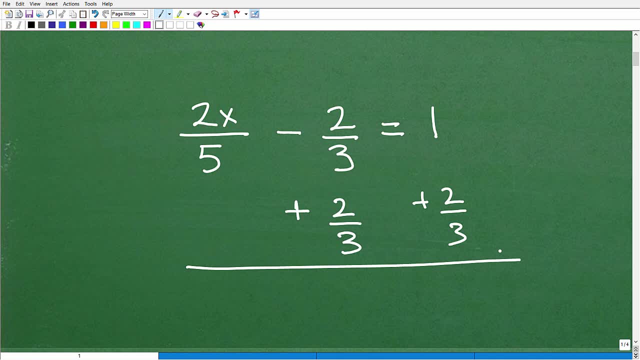 All right, And we can do all the number crunching and 1 plus 2 thirds, So then we'd end up with 2 fifths x over here And then we have 1 plus 2 thirds is 1 and 2 thirds. 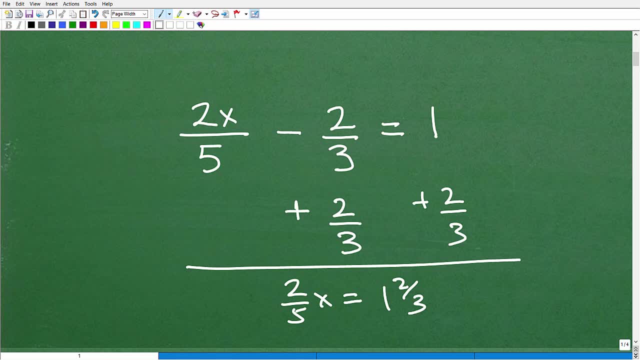 And we can kind of go from that route And then we can kind of solve. You need to know how to do the problem in that manner as well, But what I'm going to show you here is just a way that we can just kind of more cleanly, more efficiently do this problem. 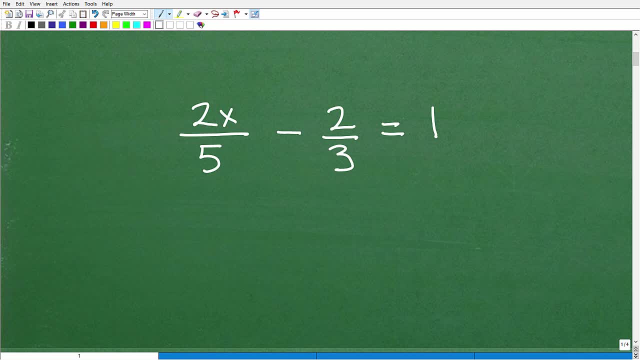 Okay, This is the way I'm going to teach my students, after I taught them more the long way. Okay, All right. So first of all, I'm like you. I don't want to be dealing with Fractions, Okay. 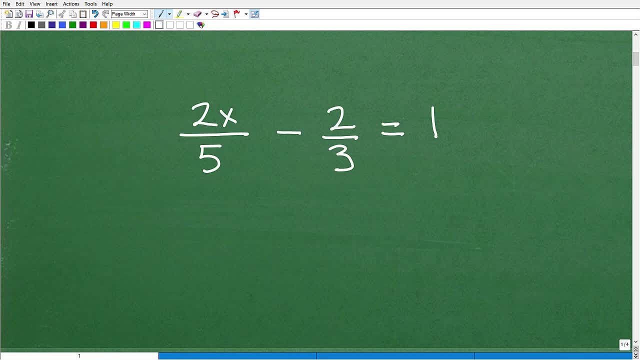 If I can get rid of those fractions, I want to get rid of them, All right. So how can I get rid of the fractions in this equation? All right, So I don't want to be mean to fractions, But you know we could be like: all right, let's just get rid of these fractions. 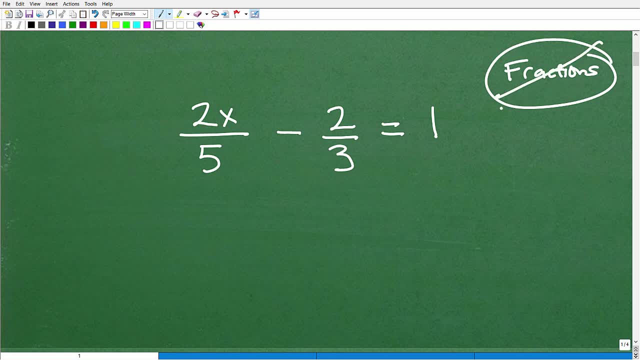 You know. you know, maybe we get a little bumper sticker put it on our car: We're against fractions. I'm not against fractions, Fractions are awesome, But you know they're kind of cumbersome to work with, Right? 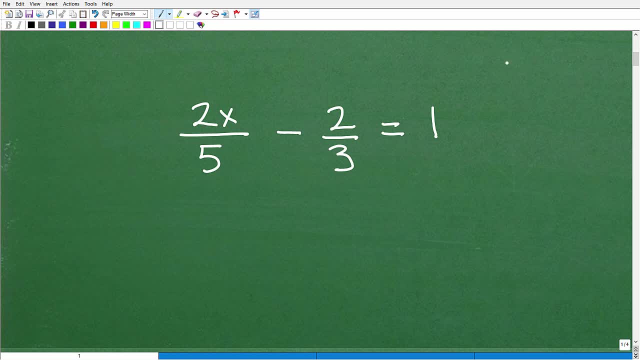 So how can I get rid of the fractions here? Well, we're going to use that trustee concept. We're going to use that the LCD. Okay, We're going to think about the LCD. Like what do you mean? the LCD? 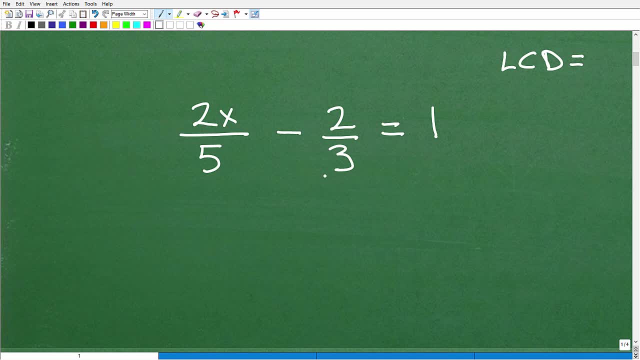 We're not. This is an equation. We're not adding or subtracting fractions. Well, if we know the LCD, this can help us clear out the fractions. So what is the LCD here? Okay, Of all the fractions involved, Well, I have a five. 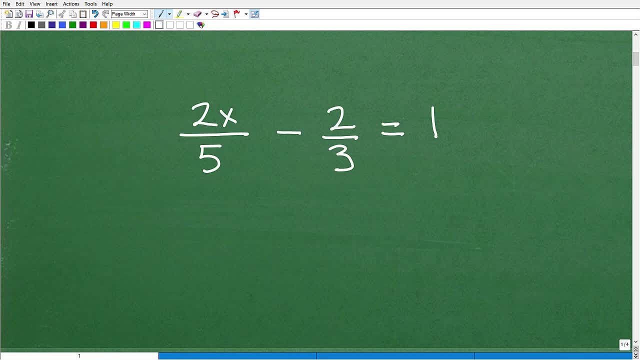 If I can get rid of those fractions, I want to get rid of them, All right. So how can I get rid of the fractions in this equation? All right, So I don't want to be mean to fractions, But you know we could be like: all right, let's just get rid of these fractions. 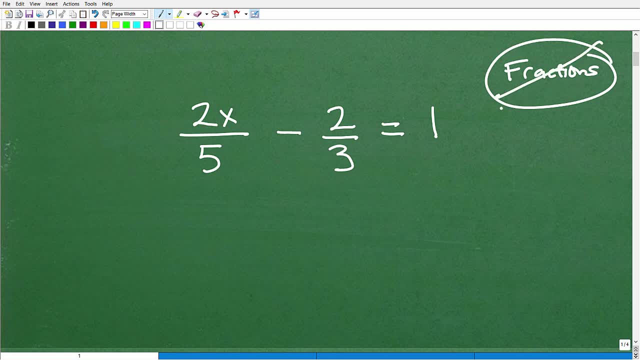 You know. you know, maybe we get a little bumper sticker put it on our car: We're against fractions. I'm not against fractions, Fractions are awesome, But you know they're kind of cumbersome to work with, Right? 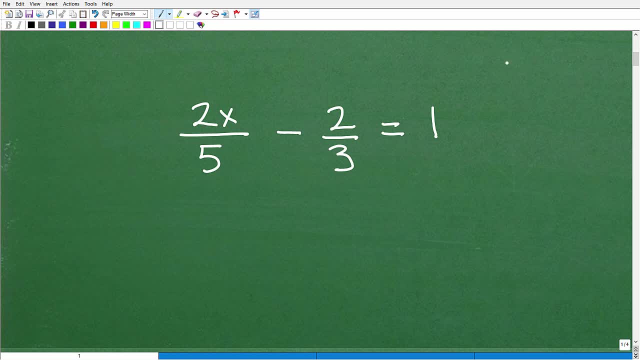 So how can I get rid of the fractions here? Well, we're going to use that trustee concept. We're going to use that the LCD. Okay, We're going to think about the LCD. Like what do you mean? the LCD? 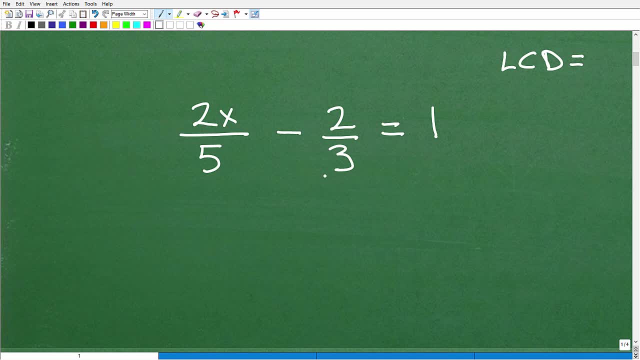 We're not. This is an equation. We're not adding or subtracting fractions. Well, if we know the LCD, this can help us clear out the fractions. So what is the LCD here? Okay, Of all the fractions involved, Well, I have a five. 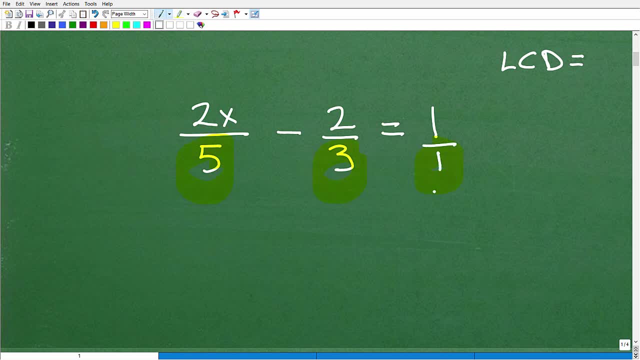 I have a three And then over here that's just one or one over one. Okay, So I have to consider all these various little denominators And I got to say, okay, what is the LCD of those denominators? It would be what you set it correctly. 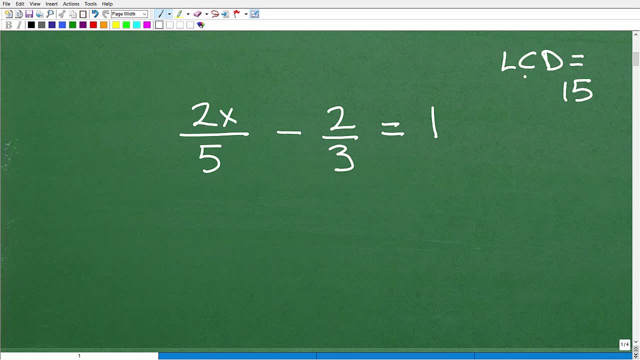 It's 15.. I know all of you are like: oh yeah, that's 15.. If you don't know how to find the LCD, then you got to really know how to you know do this correctly, All right. 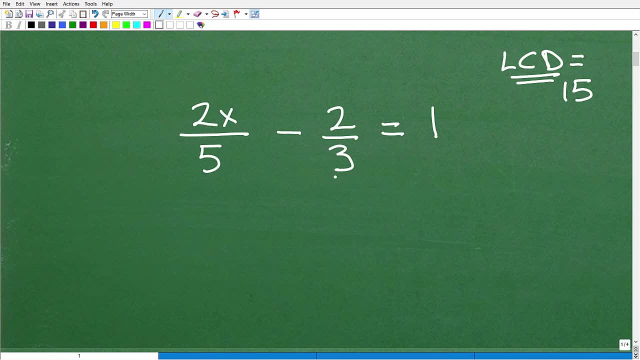 I have another video on how to find the LCD, not only with numbers but with when there's variables involved as well. Many students, you know, with a basic problem like this Can tell me what the LCD is. But if I start making the numbers more complex and I throw in some other variable situations, then they, you know, start coming up with like the wrong answers or like I don't know what to do. 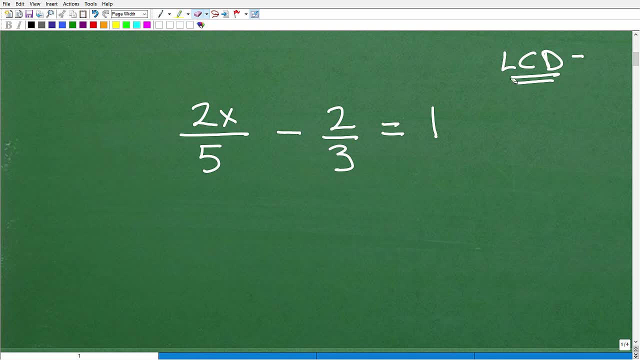 Okay, That's not good. All right So, but of course we're going to just keep it simple for the illustrations of learning how to do this. All right, So the LCD is 15.. Okay, So what do I do with this? 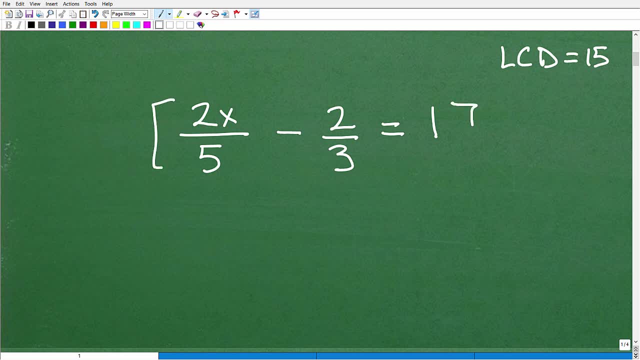 Well, we're going to multiply the entire equation by the, The LCD. Okay, Now remember in algebra: Okay, I can multiply an equation by any number or divide an equation by pretty much any number without hurting the equation. Okay, 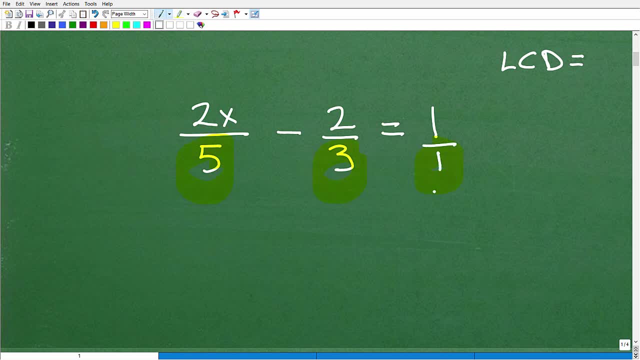 I have a three And then over here that's just one or one over one. Okay, So I have to consider all these various little denominators And I got to say, okay, what is the LCD of those denominators? It would be what. you said it correctly. 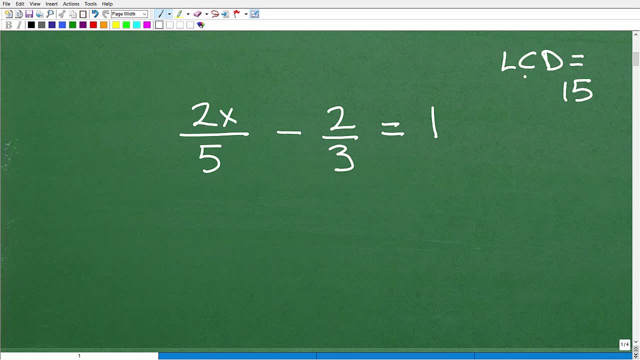 It's 15.. I know all of you are like: oh yeah, that's 15.. If you don't know how to find the LCD, then you got to really know how to you know do this correctly, All right. 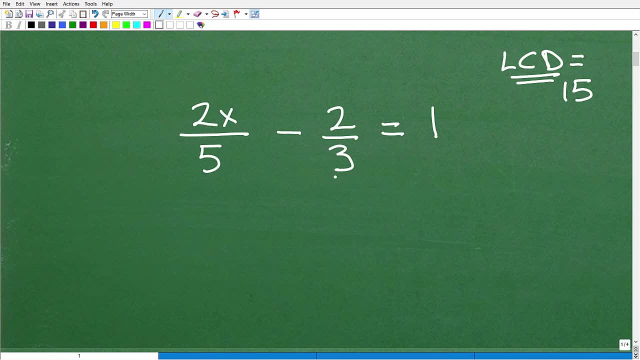 I have another video on how to find the LCD, not only with numbers, but with when there's variables involved as well. Many students with a basic problem like this Can tell me what the LCD is. But if I start making the numbers more complex and I throw in some other variable situations, then they, you know, start coming up with like the wrong answers or like I don't know what to do. 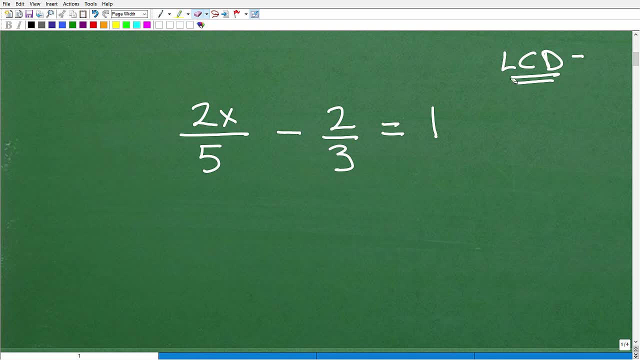 Okay, That's not good. All right So, but of course we're going to just keep it simple for the illustrations of learning how to do this. All right, So the LCD is 15.. Okay, So what do I do with this? 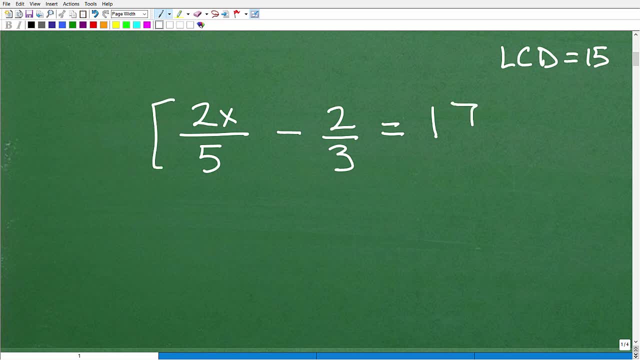 Well, we're going to multiply the entire equation by the, The LCD. Okay, Now remember in algebra: okay, I can multiply an equation by any number or divide an equation by pretty much any number without hurting the equation. Okay, 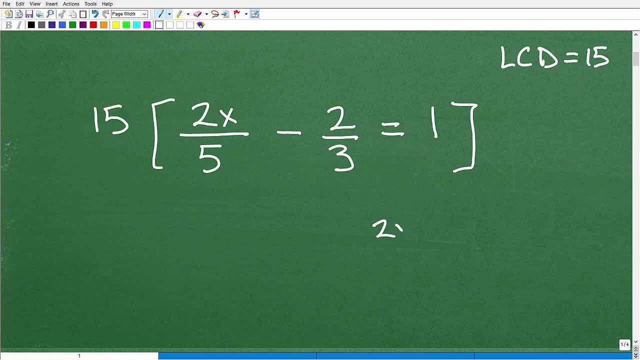 Because all you're doing is here. For example, if I had 2X equals 4 and I multiply that entire equation by 3.. Okay, I'm just going to get the new equation: 6X equals 12.. Okay. 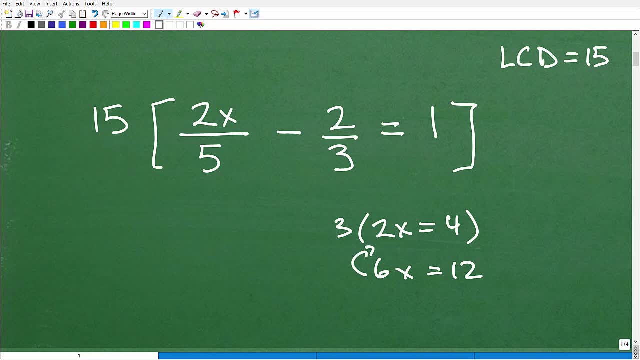 Which is The same as this equation. Okay, So you're not. you're not breaking the equation or changing the equation in any form. Okay, It's a rule in algebra: whatever we do to one side, As long as I do, whatever I'm going to do, as long as I do it to everything, then I'm going to be okay. 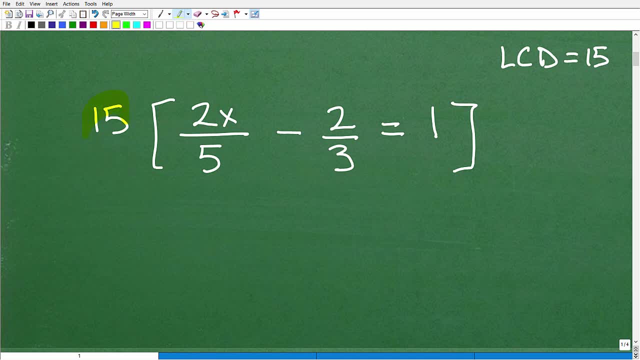 All right. So how does this help me? Okay, So here's my LCD and I'm going to multiply this by each term. Okay, All right. Now, when I do that, let's see here 15.. 15 times 2X over 5.. 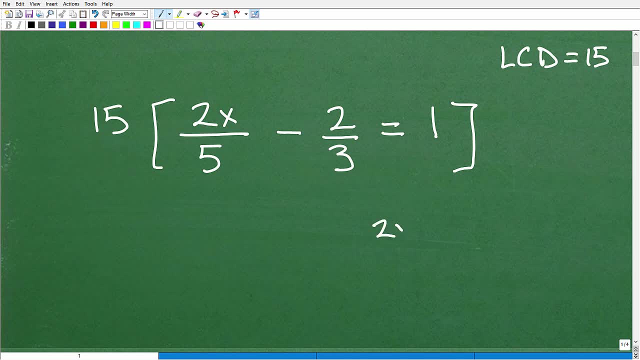 Because all you're doing is here. For example, if I had 2X equals 4 and I multiply that entire equation by 3.. Okay, I'm just going to get the new equation: 6X equals 12.. Okay, Which is? 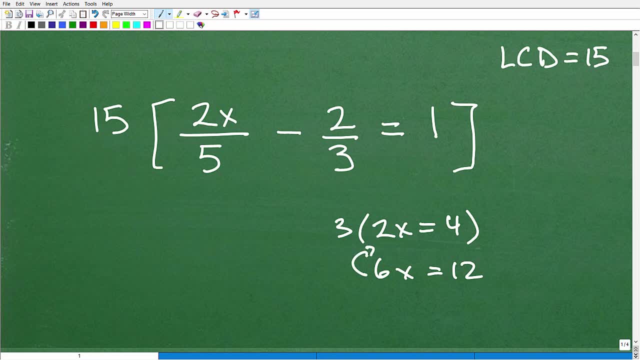 The same as this equation. Okay, So you're not. You're not breaking the equation or changing the equation in any form. Okay, It's a rule in algebra: Whatever we do to one side, As long as I do, whatever I'm going to do, as long as I do it to everything, then I'm going to be okay. 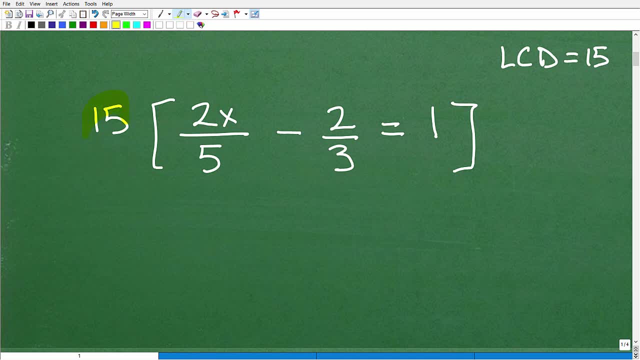 All right. So How does this help me? Okay, So here's my LCD, and I'm going to multiply this by each term. Okay, All right. Now, when I do that, let's see here: 15.. Times 2X over 5.. 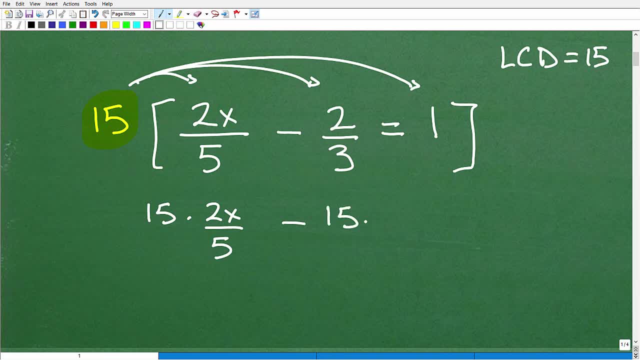 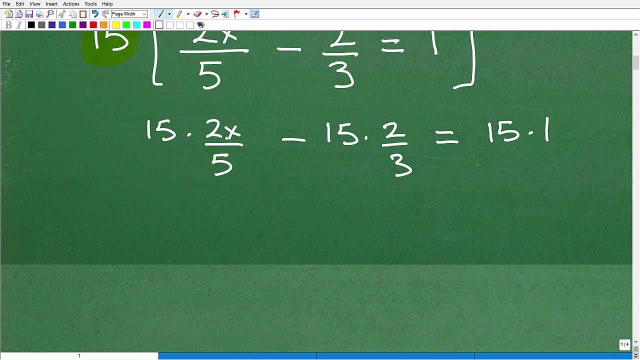 All right, Minus 15 times 2 thirds. All right, Equals 15 times 1.. Okay, So let me scroll down here. All right, So 15 times 2X over 5.. Excuse me, It's going to be what? 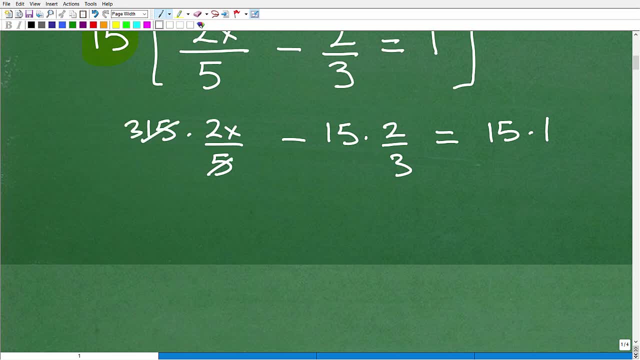 Well, 5 goes into 15.. 3. So 3 times Uh, 2X is going to be 6X, or you can went 15 times 2. That's 30 divided by 5. That's 6X minus 3 goes into 15, right here. 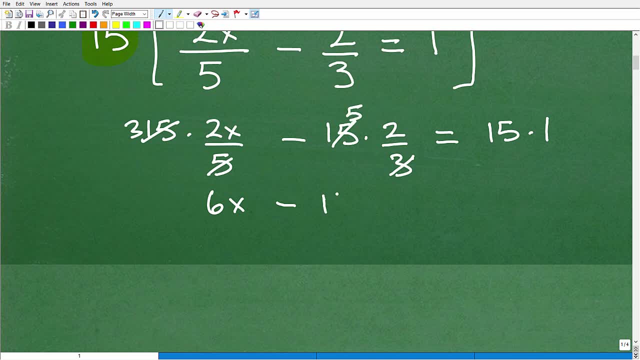 Uh, that's going to be 5.. So 5 times 2 is 10, or 15 times 2 is 30. divided by 3 is 10, equals 15 times 1 is 15.. Okay, So now I just by multiplying. 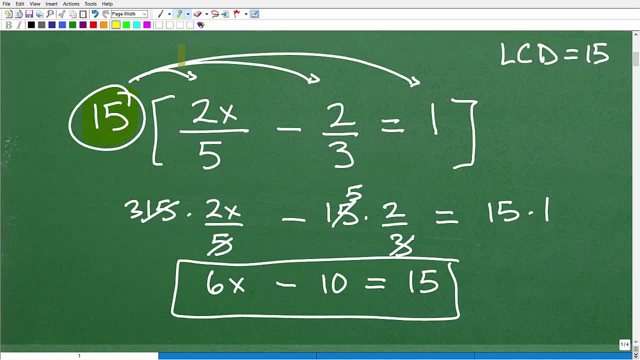 By the LCD. Okay, I was able to go from this equation here to this equation here. Okay, And there are equivalent, Okay. So you know, ask yourself, Hey, what would you rather do? Would you rather solve this guy, or rather, solve this guy? 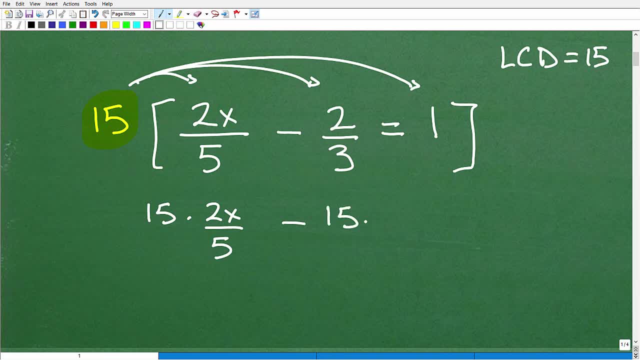 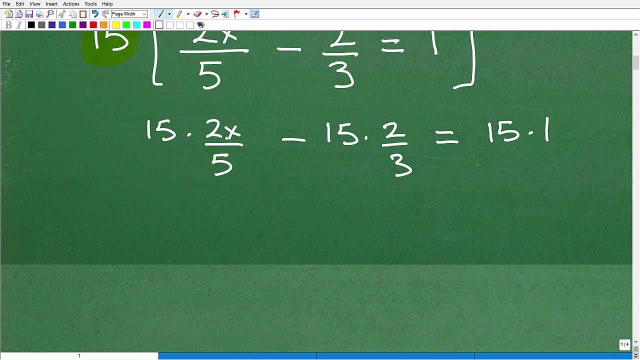 All right, Minus 15 times two thirds. All right, Equals 15 times 1.. Okay, So let me scroll down here. All right, So 15 times 2X over 5.. Excuse me, It's going to be what? 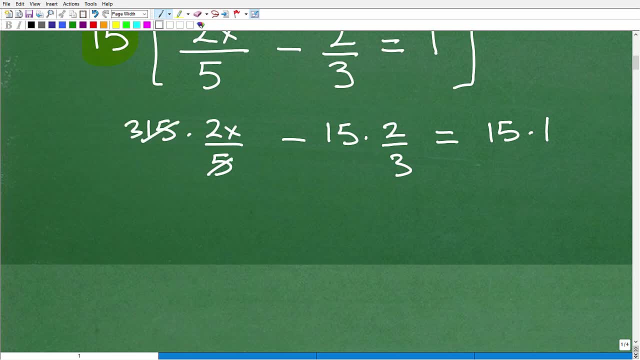 Well, 5 goes into 15.. 3. So 3 times Uh, 2X is going to be 6X, or you can went 15 times 2. That's 30 divided by 5. That's 6X minus 3 goes into 15, right here. 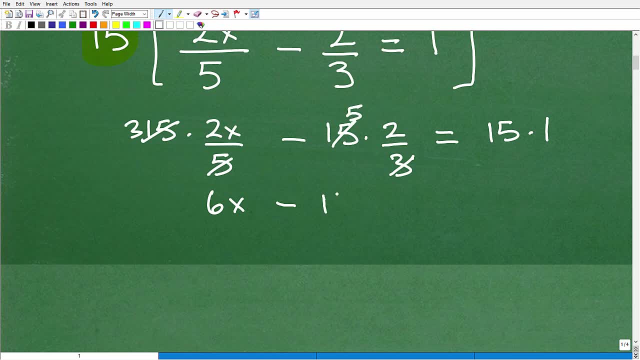 Uh, that's going to be 5.. So 5 times 2 is 10, or 15 times 2 is 30. divided by 3 is 10, equals 15 times 1 is 15.. Okay, So now I just by multiplying by the LCD. 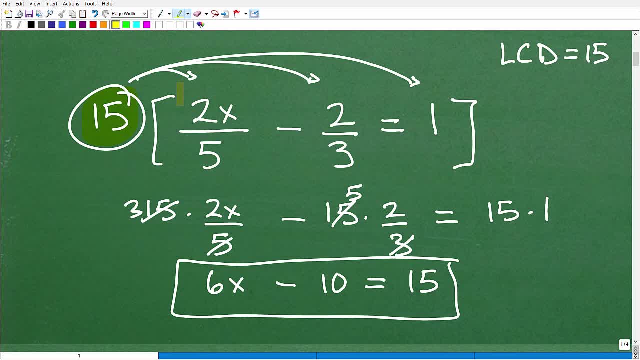 Okay, I was able to go from this equation here to this equation here. Okay, And there are equivalent, Okay. So you know, ask yourself, Hey, what would you rather do? Would you rather solve this guy, or rather, solve this guy? 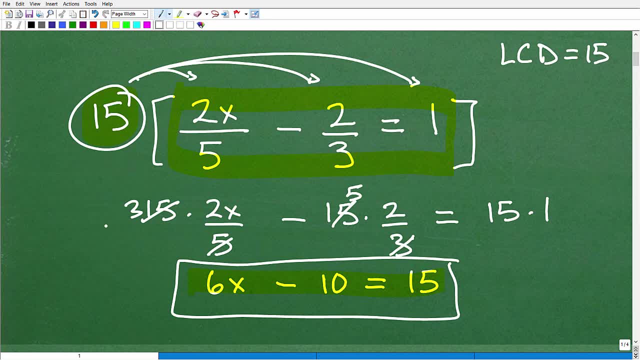 Okay, So multiplying by the LCD is, uh, by far, uh, the best approach, uh, to deal with these fractions right up front. Okay, We clear them out And now we simply can go ahead and solve for X here. 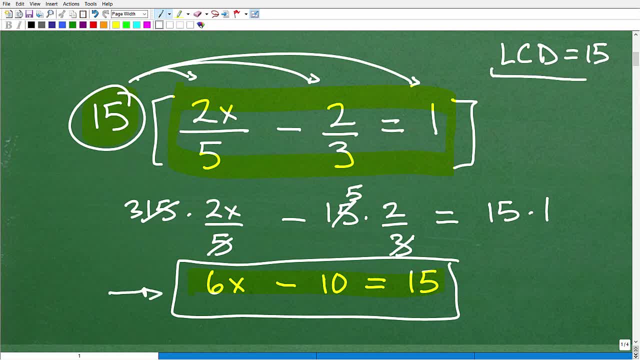 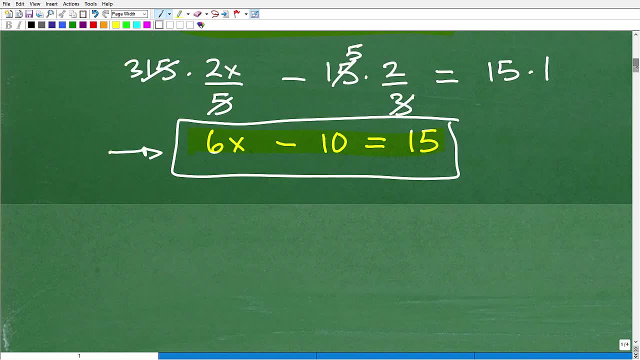 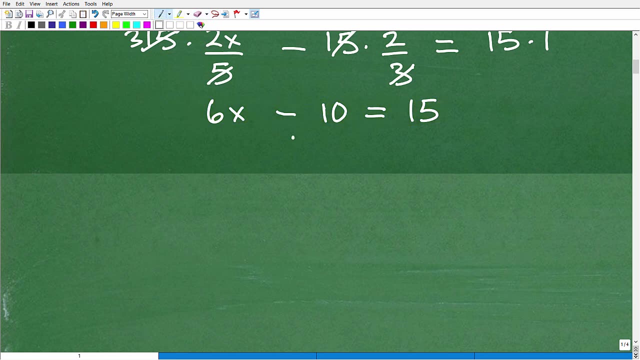 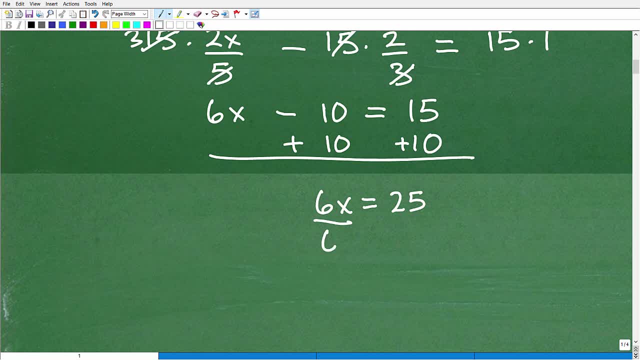 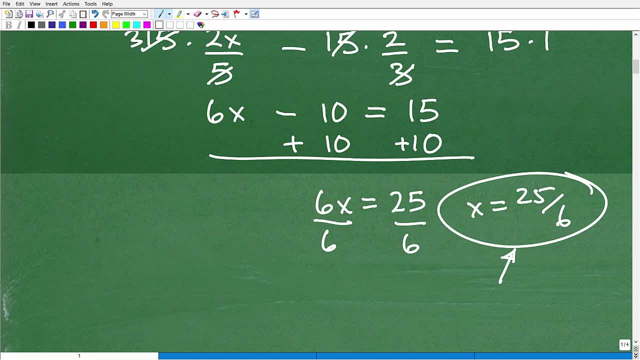 improper fraction form. because, again, if you take this into a mixed number, in other words, you go: okay, six goes into 25, that's four, and you start doing all this mumbo jumbo to write this as a mixed number. you need to know how to do that. i'm not saying that: okay, you need to know how to write. 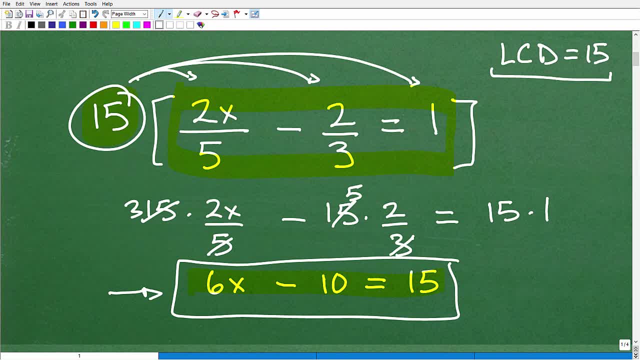 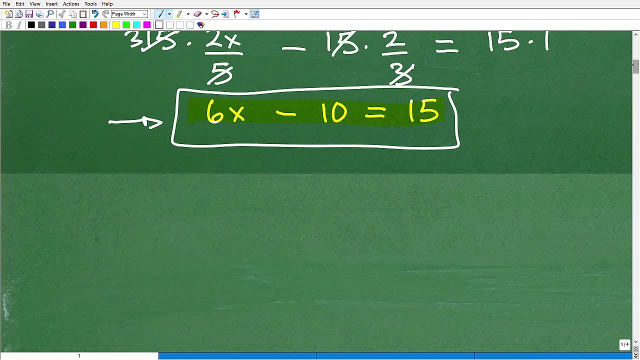 Okay, So multiplying by the LCD is by far the best approach to deal with these fractions right up front. Okay, We clear them out, And now we simply can go ahead and solve for X here. Okay, So I'm going to divide. I'm sorry. add 10 to both sides of the equation and just finish. 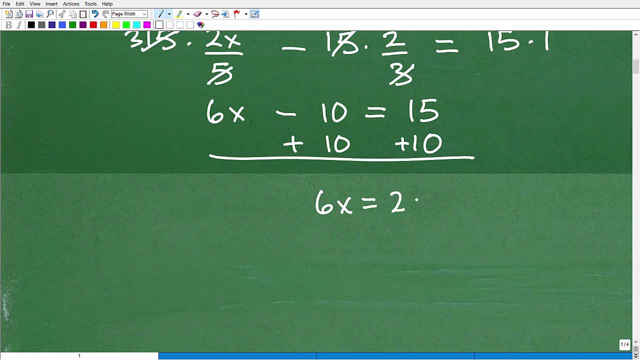 this guy up. So this is going to be: 6X is equal to 25.. And then I'm going to go ahead and divide both sides of the equation by 6.. So X is equal to 25 over 6.. And if you've been following me for quite some time, I always suggest that you do not. 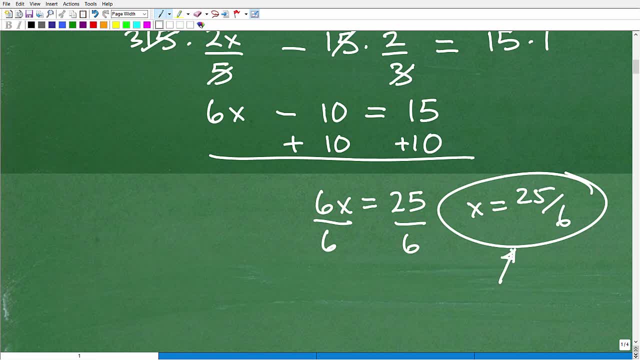 turn your improper fractions into a mixed number. Just make sure they're fully simplified, Unless your teacher or test or quiz explicitly tells you to do so. Okay, So just leave it as an improper fraction form because, again, if you take this into a mixed 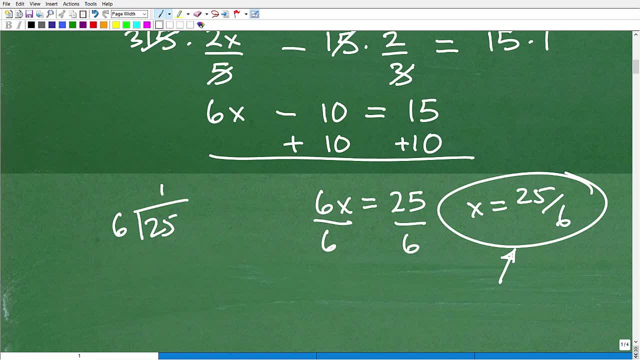 number. in other words, you go: okay, six goes into 25.. That's four And you start doing all this mumbo jumbo to write this as a mixed number. You need to know how to do that. I'm not saying that. 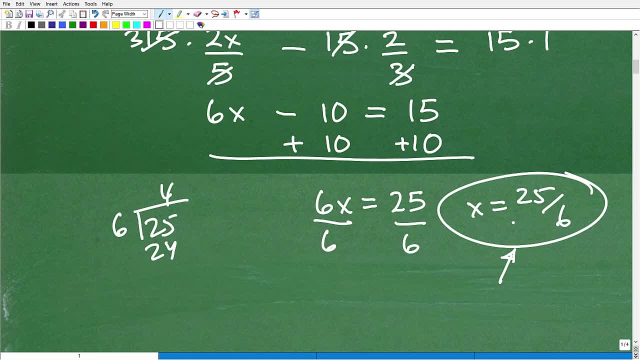 Okay, You need to know how to write a improper fraction as a mixed number, but this requires time and additional work And it also requires time And it also increases the probability of you making an error. Okay, I've seen countless times where students have the right answer as improper fraction. 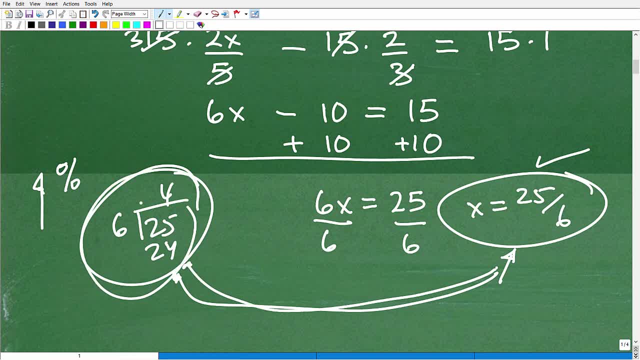 Then they go do all this extra work and then they make a mistake and then give me the wrong answer. They're like: oh, it's four and two sevenths or something like that, And now I got to take points away from them. 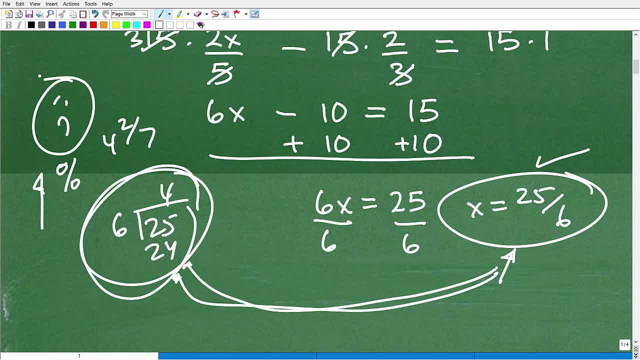 And I, you know, then there's a sad face. Okay, We don't want that situation. So again, unless your teacher tells you explicitly, you know, turn all your work into a mixed number And, uh, into a mixed numbers, leave them alone. 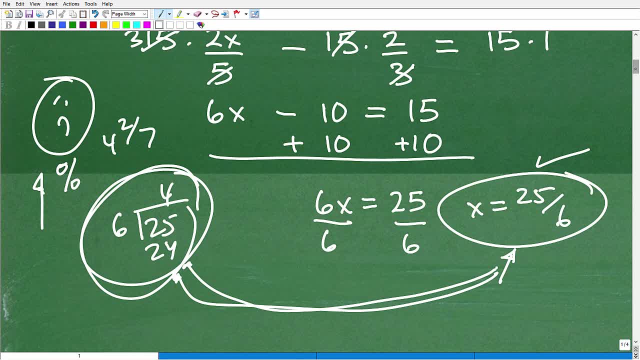 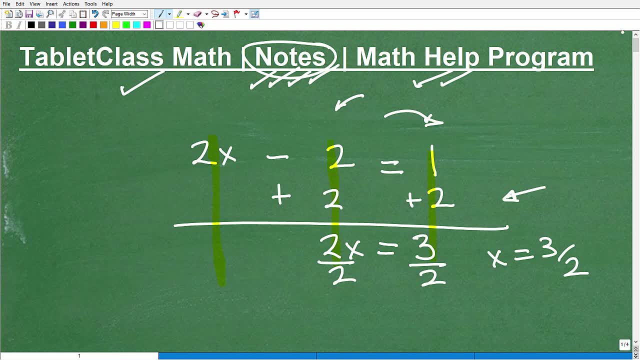 Okay, Just make sure they're fully simplified. Okay, So again, you know when you're faced with the problem. okay, Basic algebra problems. you got to make sure you know just the. uh, you know one and 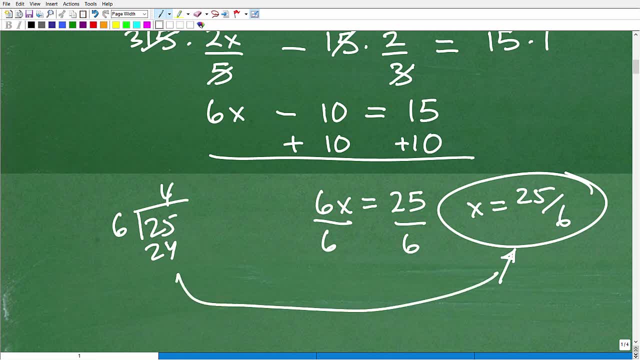 a improper fraction as a mixed number. but this requires time and additional work and it also increases the probability of you making an error. okay, i've seen countless times where students have the right answer as improper fraction. then they go do all this extra work and then they make. 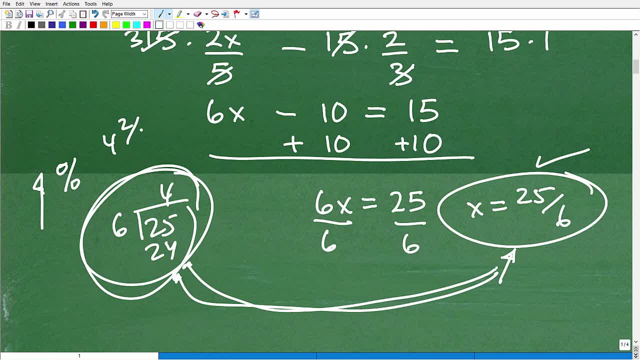 a mistake and they give me the wrong answer. they're like: oh, it's four and two sevenths or something like that, and now i got to take points away from them and i you know, then there's a sad face. okay, we don't want that situation. so again, unless your teacher tells you explicitly, you know. 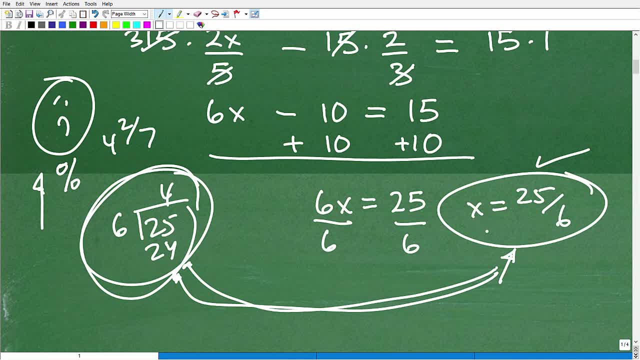 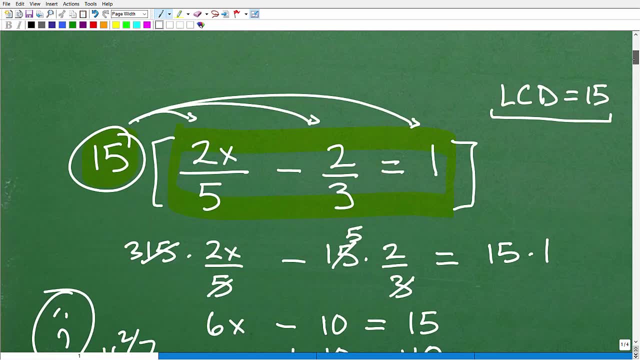 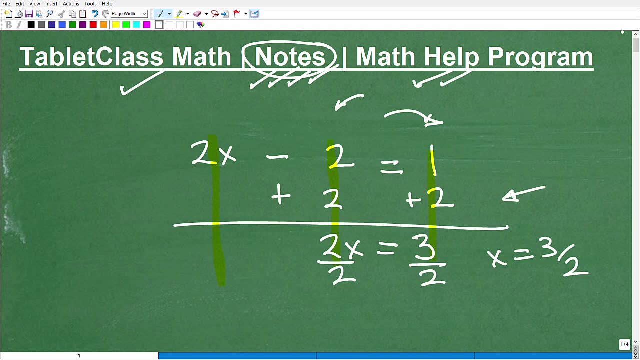 turn all your work into mixed numbers. leave them alone. okay, just make sure they're fully simplified, okay. so again, you know when you're faced with the problem. okay, basic, uh, algebra problems. you got to make sure you know just the, uh, you know one and two step, you know scenarios. now there's other approaches to solving. 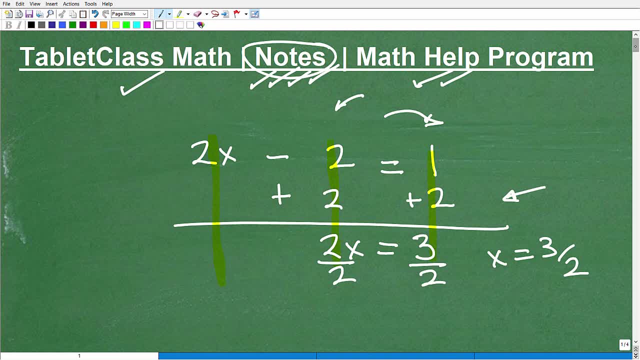 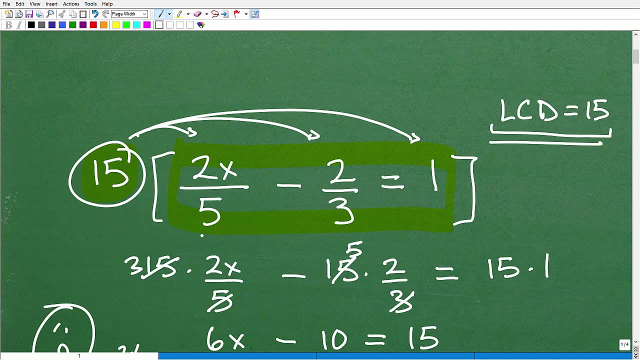 this particular problem, but using lcd to clear out fractions is is excellent, okay, and this is really comes in handy when you're doing much more advanced algebra equations. so i would suggest start practicing this concept now, but, you know, if you, you know, did this problem a different way and got the right answer. 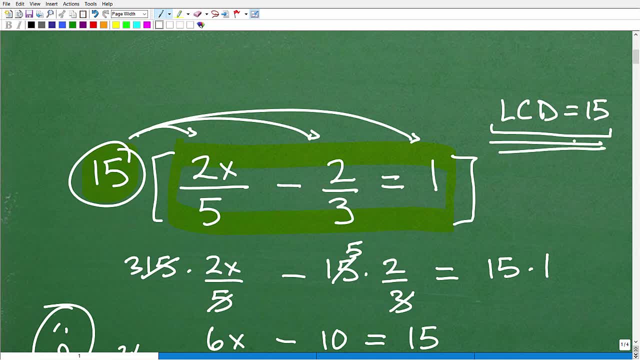 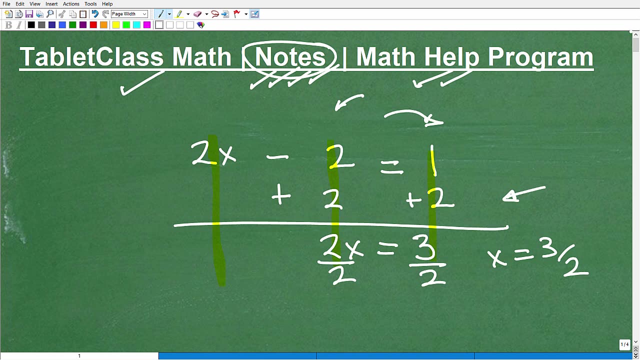 that's fine too, but you need to know how to determine what the lcd is of an equation, of all the different terms in it, and how to clear out the fractions. okay, all right. so, with that being said again, none of this is going to stick unless you practice. so you got to reinforce this if 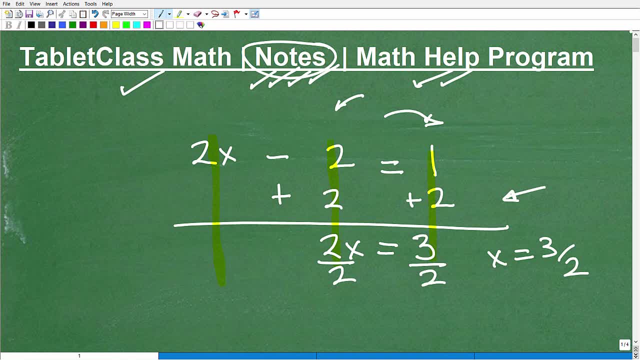 you're. you know, you know practicing by doing out your homework and algebra equations. if that's what you're studying right now, that's great, but remember, you got to practice this stuff and they also got to put this into your notes. okay, all right. so, with that being said, if you enjoyed this video, i 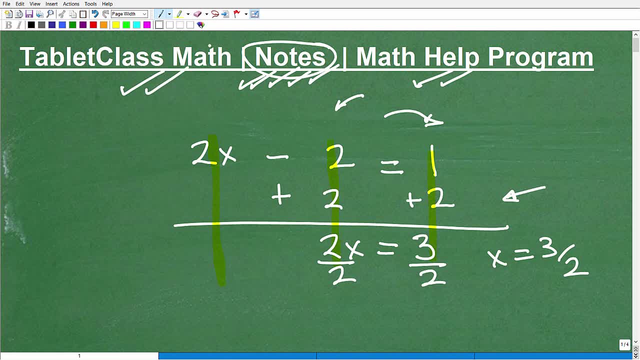 definitely appreciate a thumbs up and hopefully you- you um- will subscribe. if you are a current subscriber, i thank you for that, but i already have hundreds and hundreds of videos on my channel that can help you out. so if you're struggling in other areas of math, please check out my other.